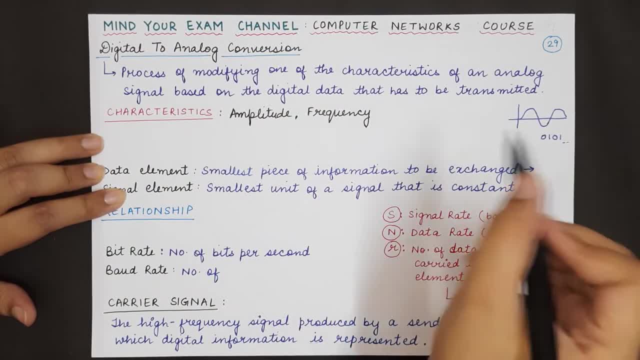 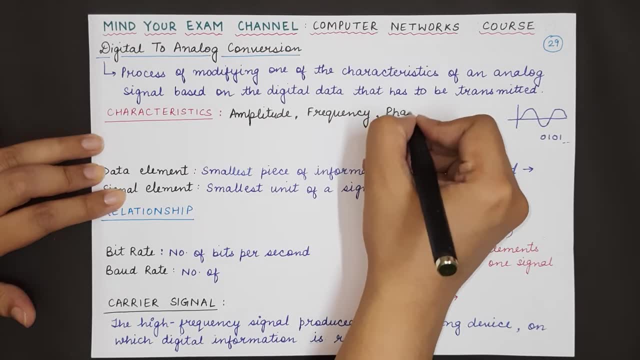 waves. how many cycles are getting completed by a signal in one signal? So the second characteristic will be the frequency: atmosphere. So an analogue signal has to be over time. unit is known as the frequency and the third one is the phase. So there are three important characteristics of any analogue. 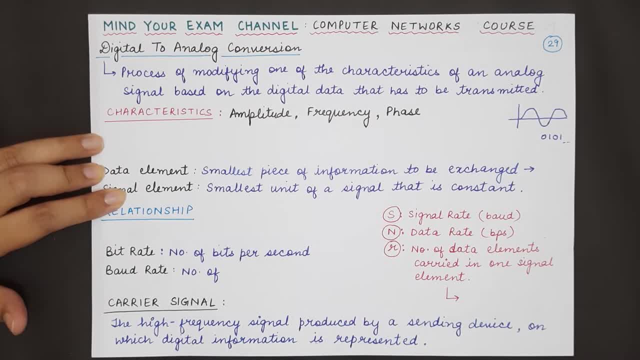 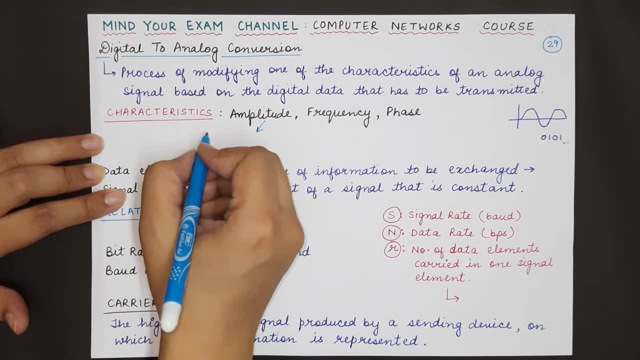 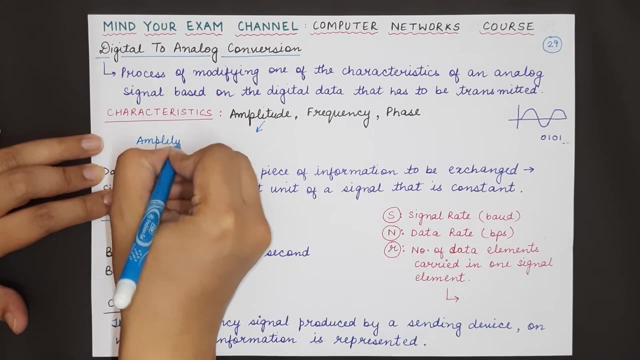 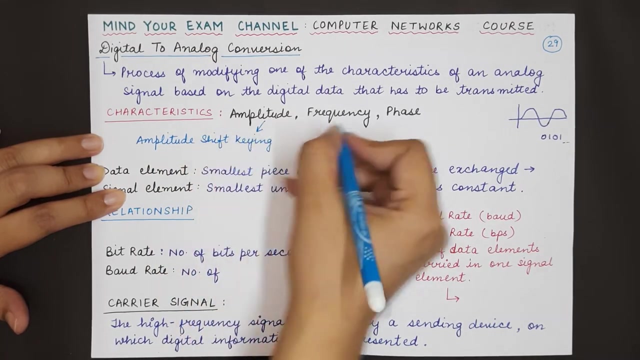 signal And by changing these characteristics you can perform digital to analog conversion. So if you change the amplitude of the analog signal to encode or represent your digital information, then that is known as amplitude shift keying. okay, change the frequency, it will be known as frequency shift keying. and if you change the phase, that 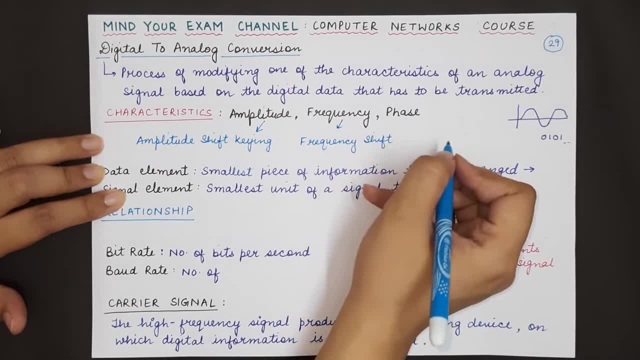 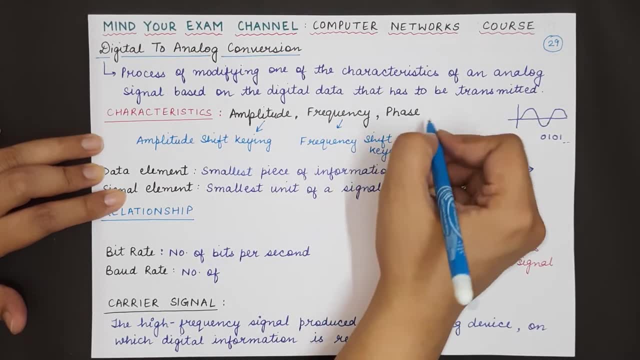 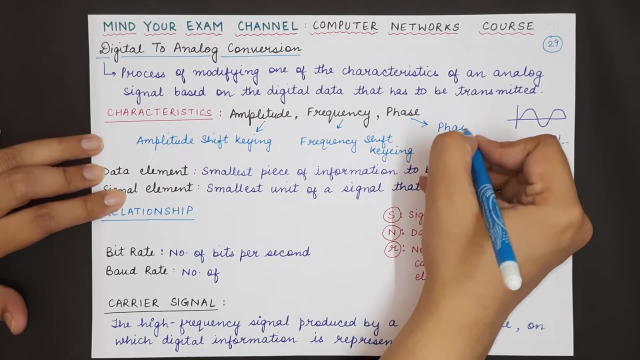 will be known as phase shift keying. okay, PSK, ASK and FSK now. shift keying basically refers to the process of changing either the frequency, amplitude or phase to represent digital information for transmission of data. okay, now, in this case, what we are basically doing. we need to. 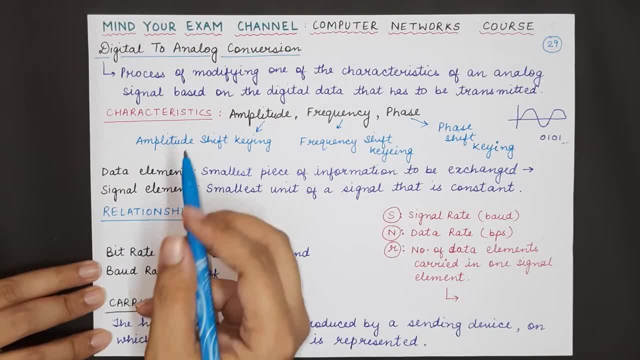 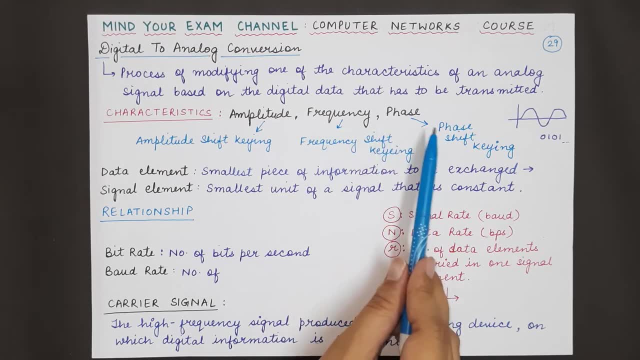 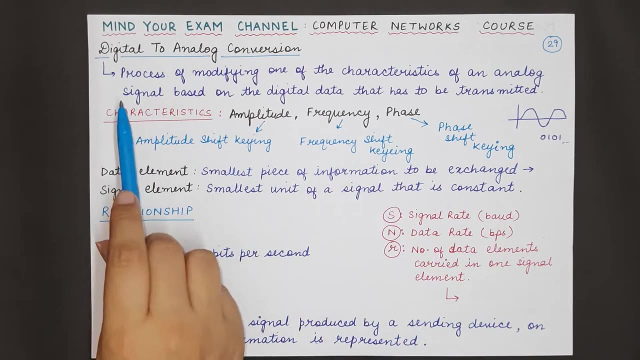 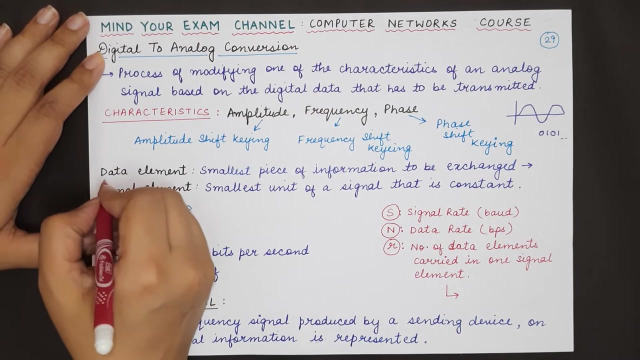 study some important terms and some important formula that will be used in future when you study each of these amplitude, frequency and phase shift keying techniques that we will be discussing in the future lectures. so for digital to analog conversion, you must know what is meant by data element. so these two terms are very important: data element and signal element. so data element. 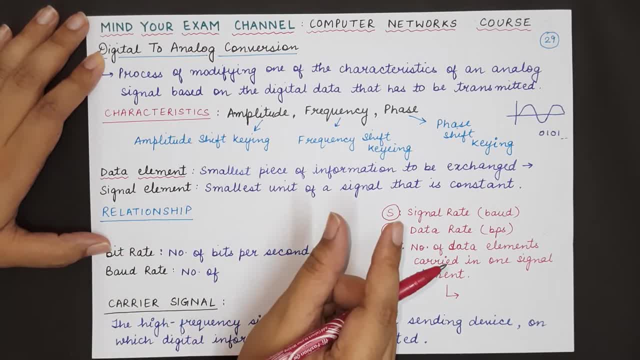 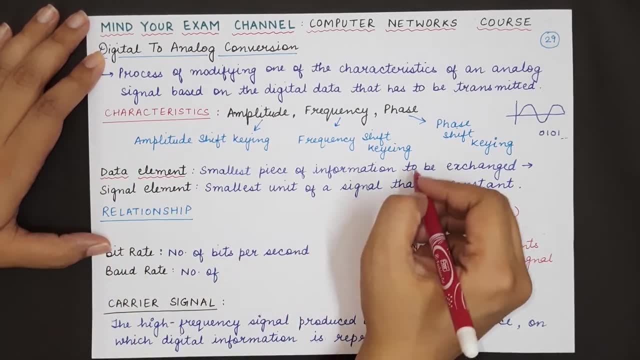 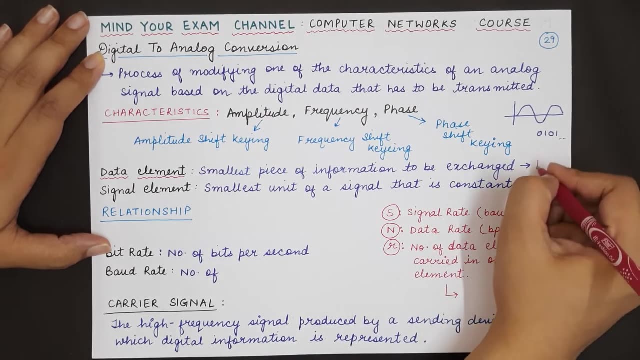 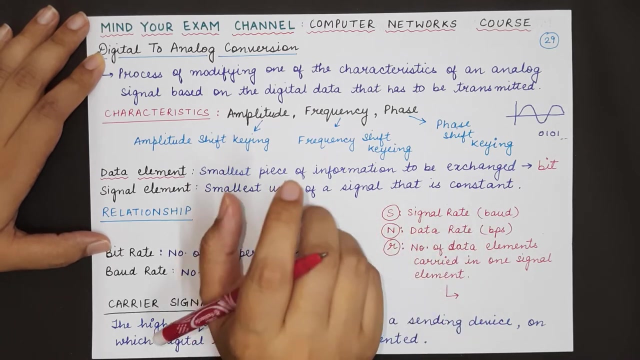 basically means the smallest unit of information that can be represented on the signal and that smallest unit of information that has to be exchanged during signal transmission. so basically, the smallest data element is the bit. okay, now, when you encode multiple bits, your smallest data element becomes the number of bits that you are encoding in each signal. 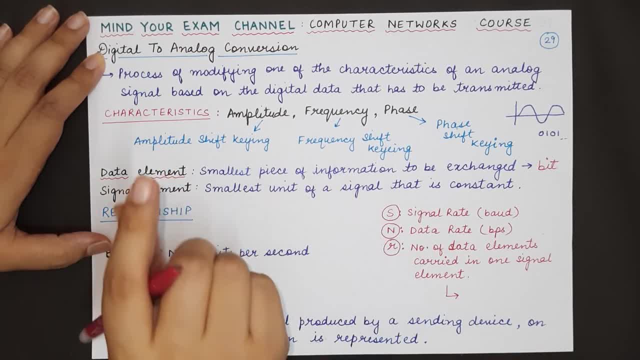 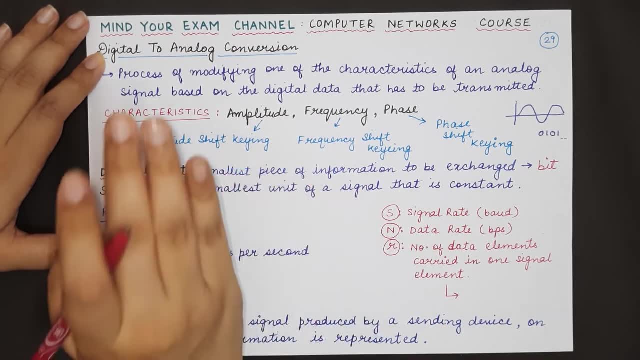 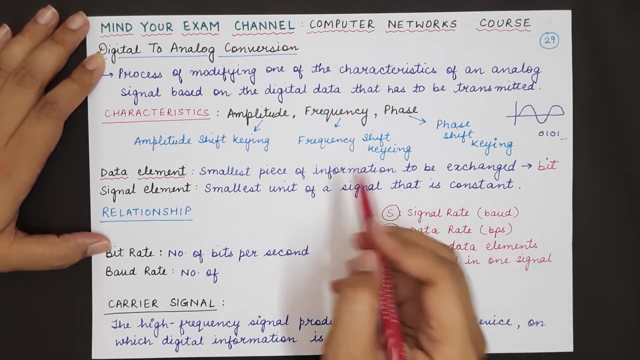 element. So if you are sending 1 bit, representing in a single signal element, then the data element will be 1 bit. If you are representing 2 bits, then that in that case the data element will be 2 bits- smallest unit of information that you are transmitting for exchange of information. ok, 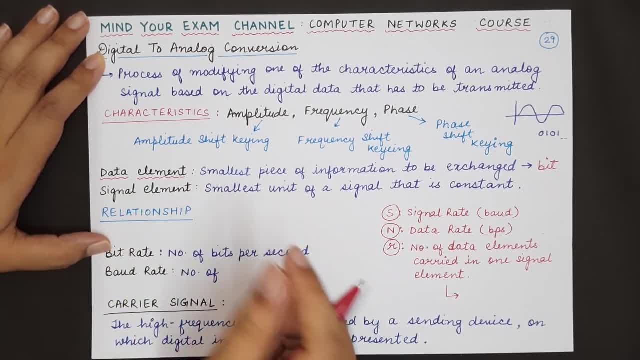 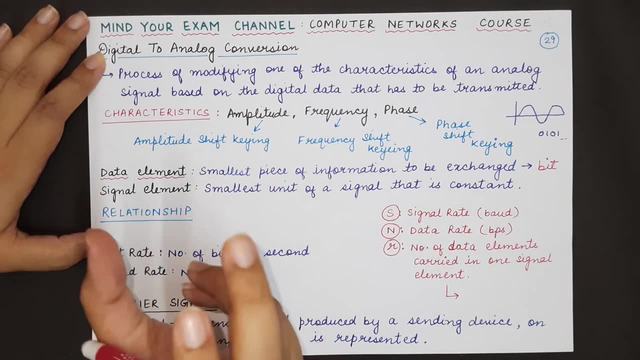 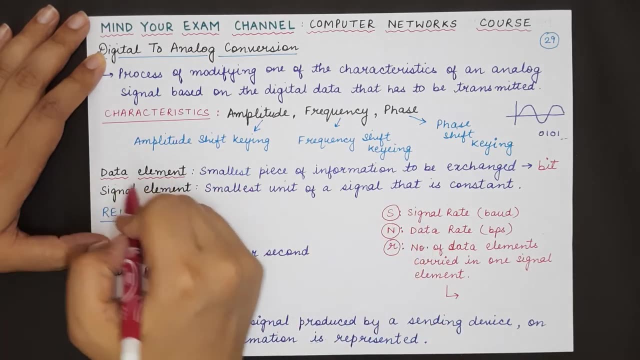 So, as I said, the signal element basically means the smallest part of the analog signal that remains constant, or that is constant, or the smallest part which eventually repeats itself, the part that actually carries the data element. ok, Now, what is the relationship between a signal element and a data element? 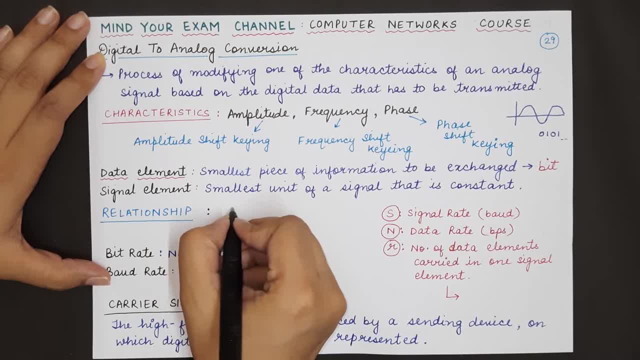 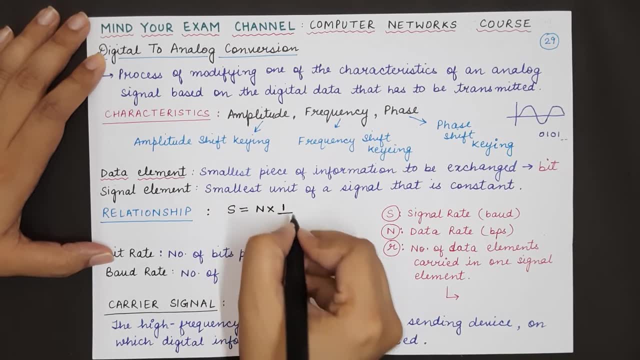 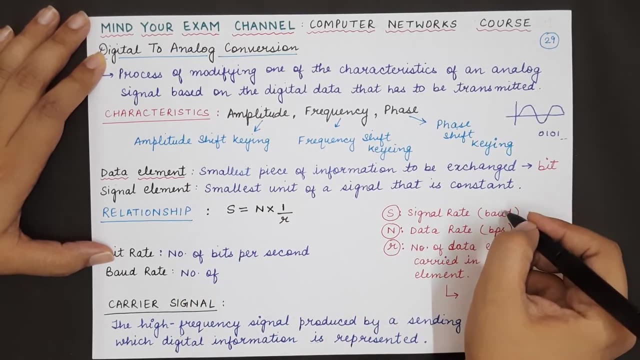 So this formula is very important. So the formula is: Signal element is equal to data element multiplied by 1, by R. Now here: S represents signal element and the unit is Baud. N represents data. sorry, S represents signal rate and the unit is Baud. 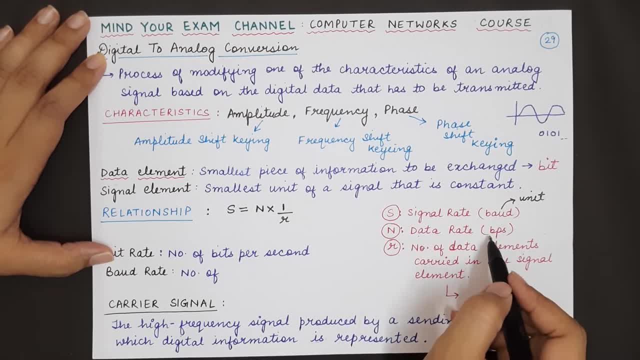 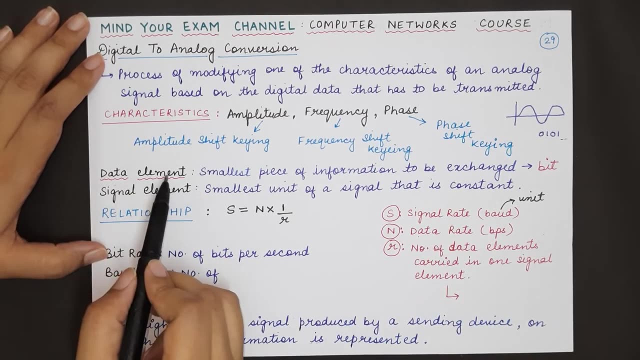 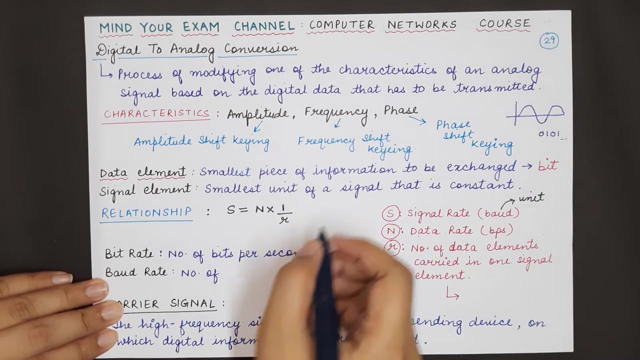 N represents data rate and the unit is bits per second, or BPS, and R represents the number of data elements. So we have understood that 1 data element basically means that the smallest unit of information that is being transmitted. So bit rate is defined as the number of bits per second that are being transmitted. and 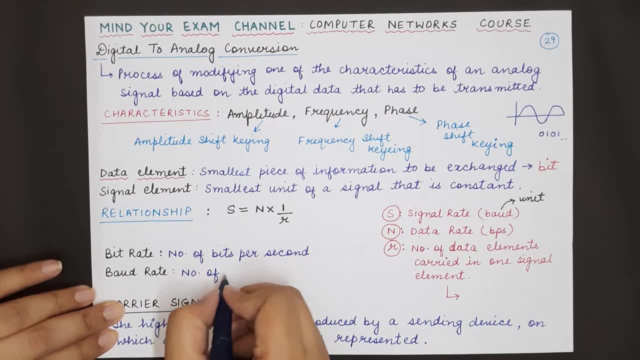 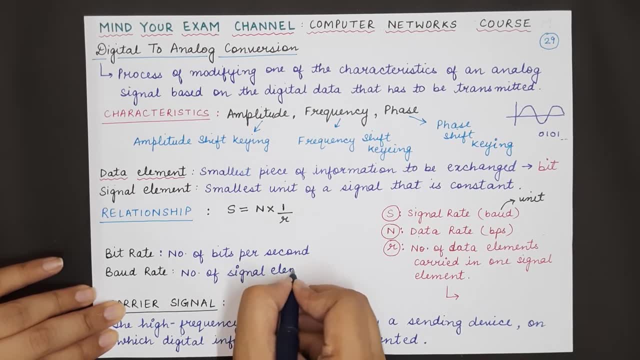 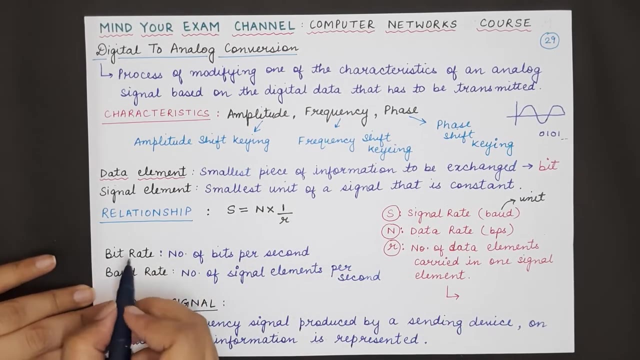 Baud rate or the signal rate specifies the number of signal elements carried in one signal element. There is two different binary elements that are being transmitted per seconds, where the elements are being transmitted to the data. So this two terms will help you understand what the bit rate that means, how many bits? 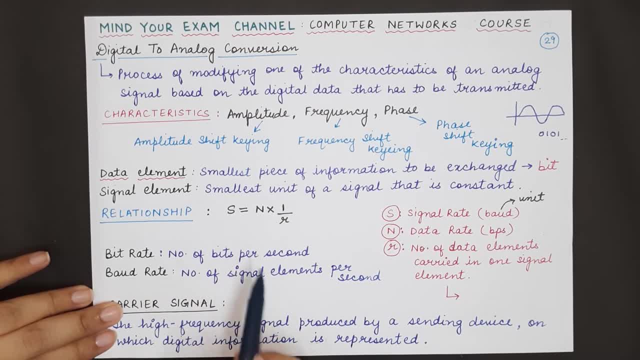 are being sent per second, and the Baud rate is how many the signal elements are traveling in the analog signal dynamic that is being transmitted. per then, Now the relationship between the bit rate and the Baud rate is represented by S- is equal to 1 by R. So the Gingerly Fadtome's results: the band light is determined in terms of the bits aberrated or nothing but, And the output of the시고. So the BRAVE regional migration And caso de la symbol is the belo n shells. 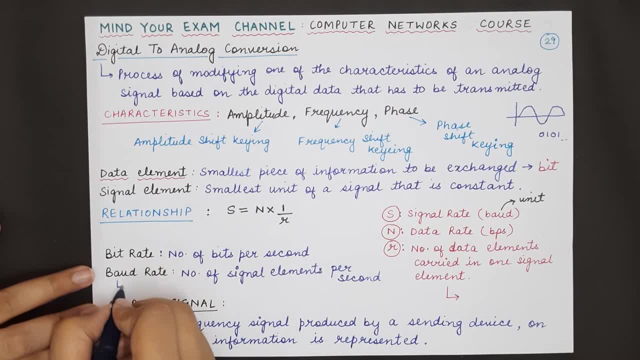 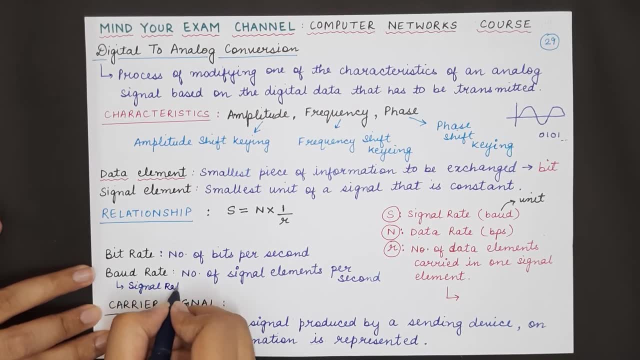 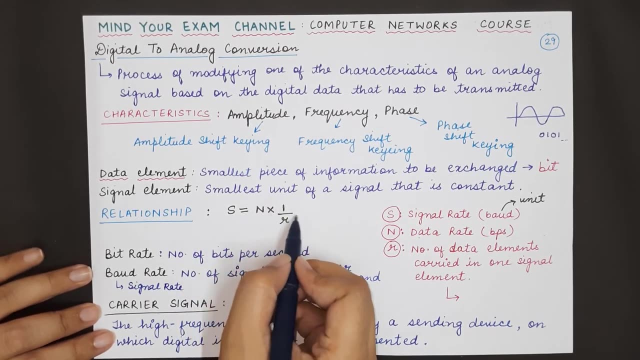 But if we identify the units of data along the diversity team driving standards, well, that's a good S. you can say either as the bit rate or the sorry, you can say it as the baud rate or the signal rate. okay, So these are used interchangeably. So signal rate is equal to data rate multiplied by 1 upon. 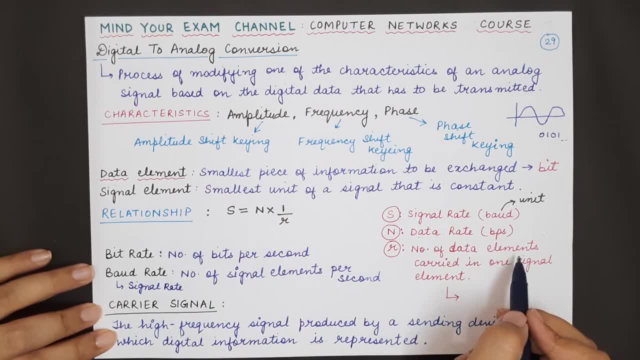 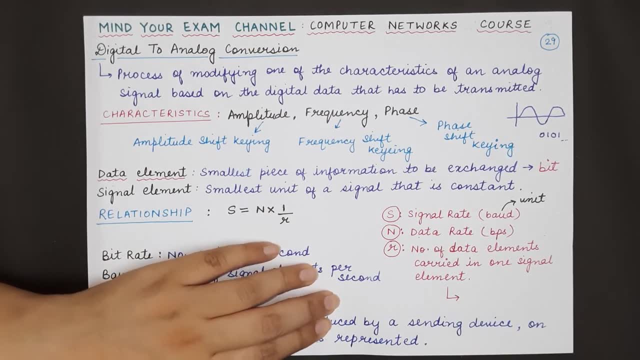 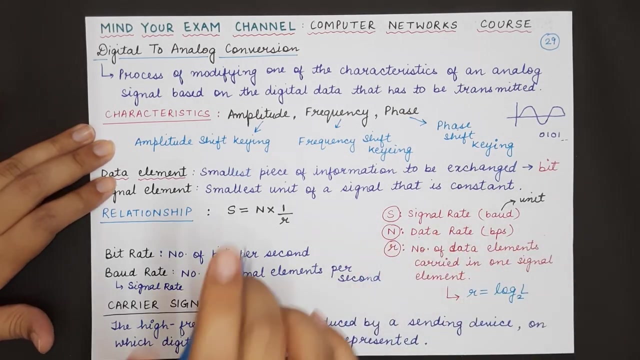 r, where r represents how many data elements are carried in one signal element, and the formula for calculating r is given by. r is equal to log l base 2, where l represents the type of signal element that is being transmitted. So the value of l would be given to you if you are performing. 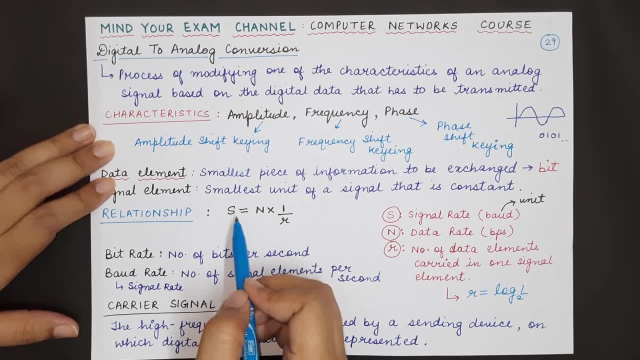 any numerical question and you have to then calculate how many signal are getting transmitted in one second by using the value of r and the data rate, Okay, or if data rate has to be calculated, then you will be given the values of s and r and you 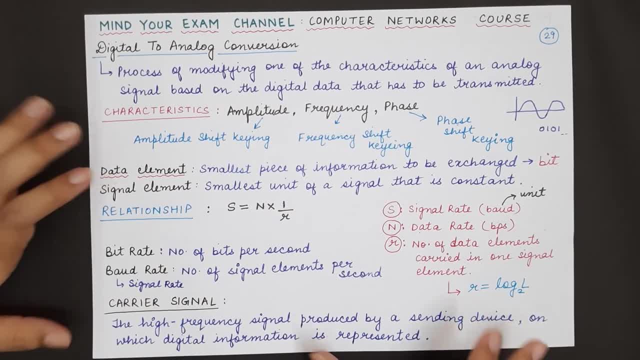 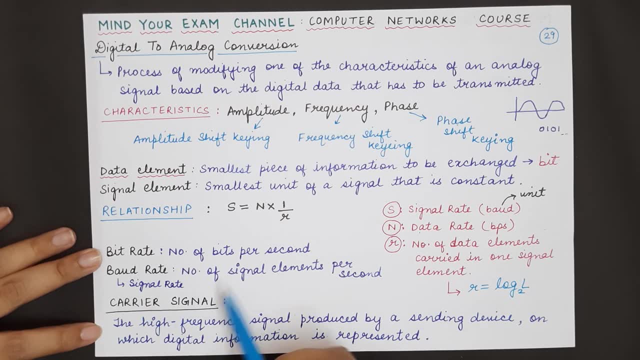 can easily calculate. Now the last and important point for this particular video is: what is a signal, carrier signal? So carrier signal is that high frequency analog signal which is produced by a sending machine so that digital information is represented on that signal. So basically, in digital to analog conversion, the signal, the analog signal that actually carries digital. 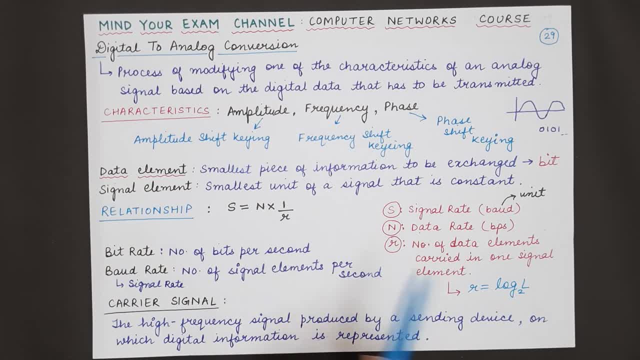 information from the sender to the receiver. that particular signal is known as the carrier signal. So it is the characteristic of the carrier signal that we are actually changing. If we change the amplitude of the character signal based on the information that we want to transmit, it becomes: 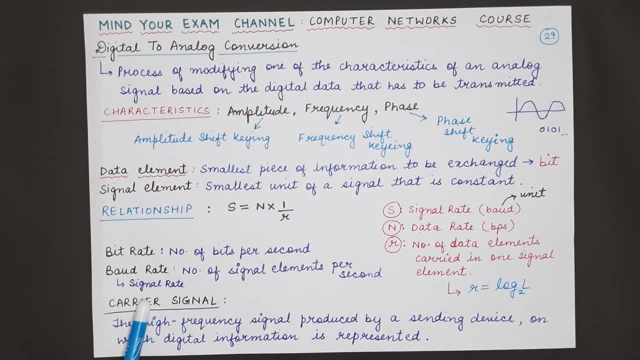 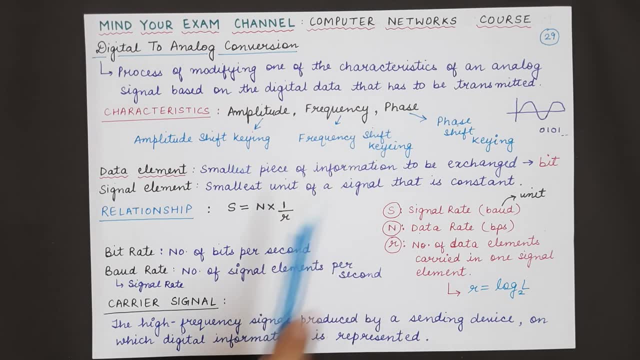 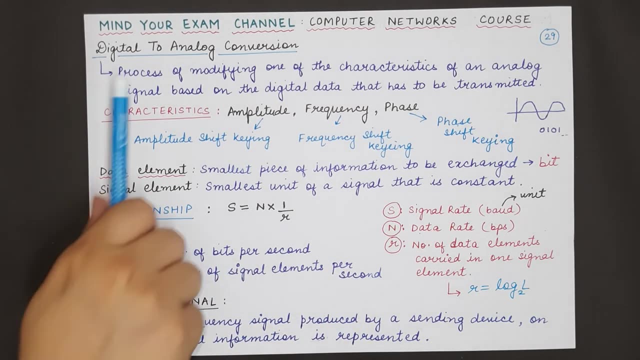 amplitude shift keying. If we change the frequency of the carrier signal based on our digital data, it becomes frequency shift keying, and if we change the phase of our carrier signal, it becomes phase shift keying. Okay, so these were the basics of digital to analog conversion. In the next video we will 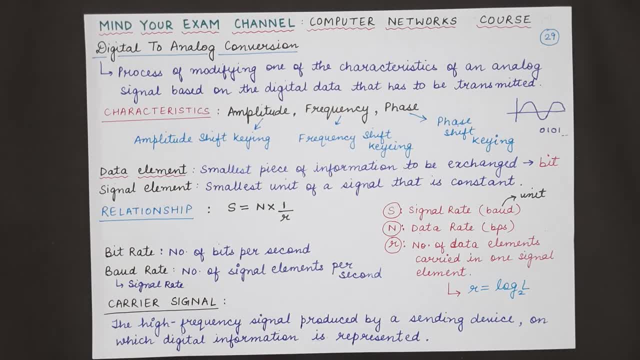 be studying about three different types of digital to analog conversion techniques, the shift keying techniques. Okay, thank you for watching. If you understood this video and it helped you in some way, please let us know in the comment section below. like our video, share with your friends and also mention if you.